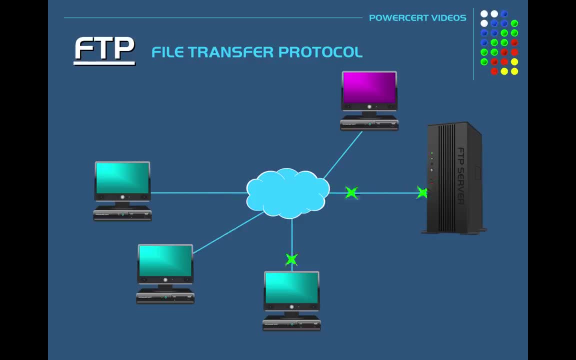 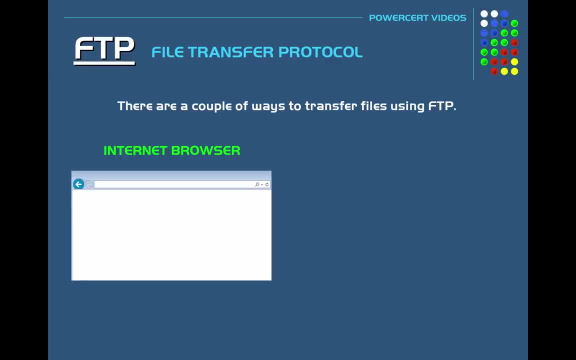 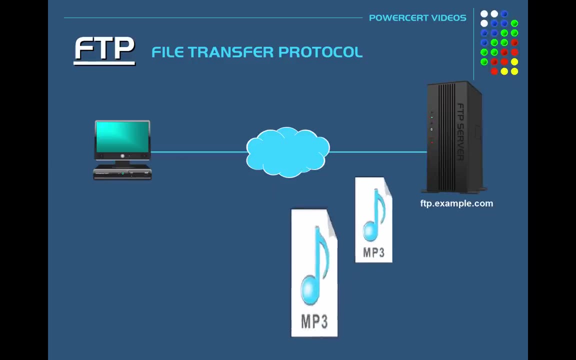 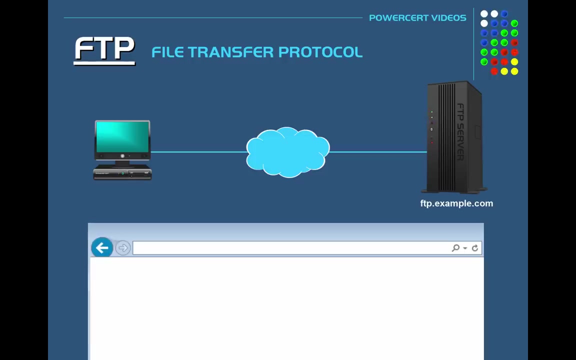 Windows. this FTP server can be used to transfer files to other computers, For example, in Microsoft Windows. this FTP server can be used to transfer files to other computers. For example, in Microsoft server is ftpexamplecom, So you would type that address as the URL Now normally if you were going. 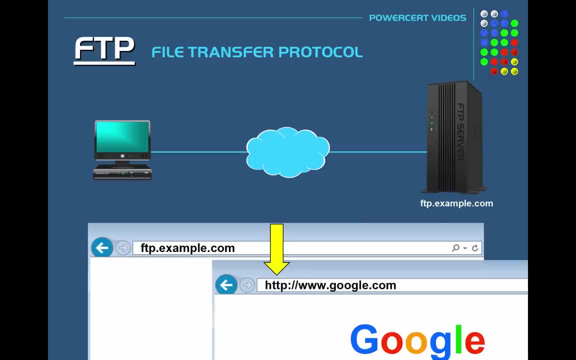 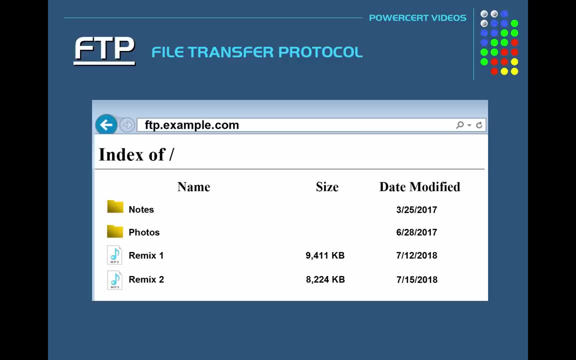 to a regular website, the prefix would be HTTP. But since we are going to an FTP site, the prefix is FTP. So now we're connected to the FTP server. So here is an example of an FTP server view in a web browser And from here you can browse different folders. that's on the FTP server. 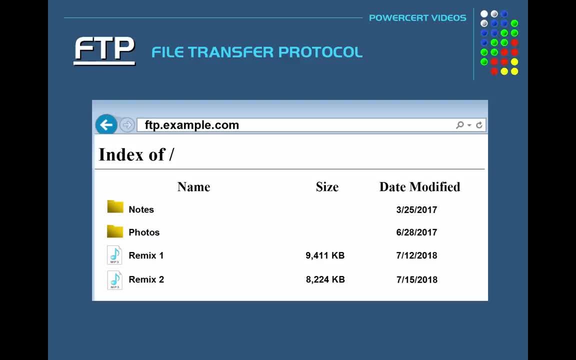 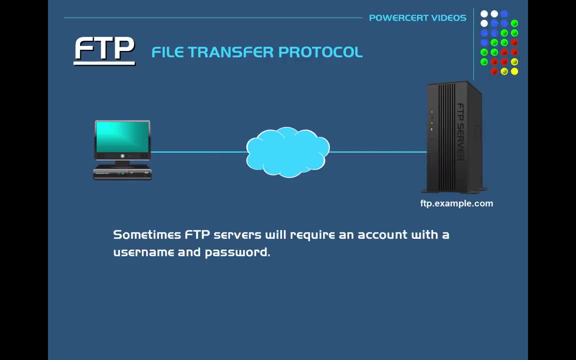 depending on what the owner has made available, and then you can view and download what you want. So here are the mp3 files, and then you can just click the files and then download them to your computer. Now, sometimes FTP servers will require an account with a username and password, and 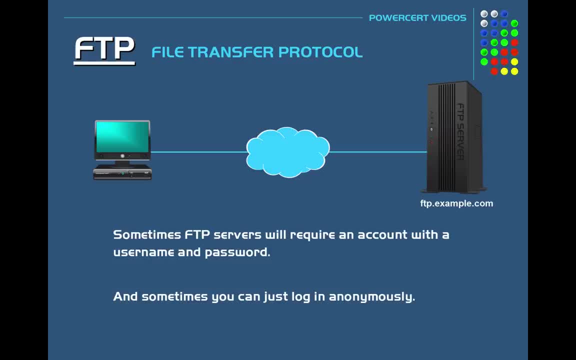 sometimes you can just log in anonymously. It just depends on what type of authentication you're using. So, for example, if you're using a web browser, you can just log in anonymously. It just depends on what type of authentication that the owner of the FTP server has set up And another way that you can connect to an FTP server. 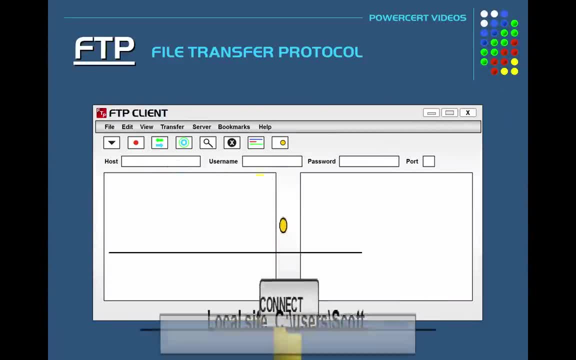 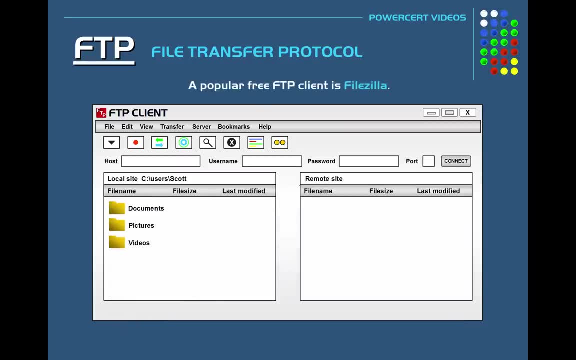 is by using an FTP client. Now, there are a number of FTP clients that you can use, but probably the most popular free FTP client is called FileZilla, which you can download for free. So here is an example of an FTP client And, as you can tell, using an FTP client provides a great 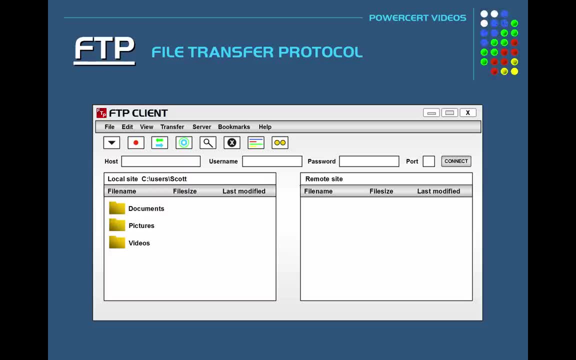 graphical user interface and a better overall experience than using a web browser. So up here is where you would provide the address of the FTP server, along with the username and password, if required, and the port number, which would be port 21.. And then you would just hit the connect button. 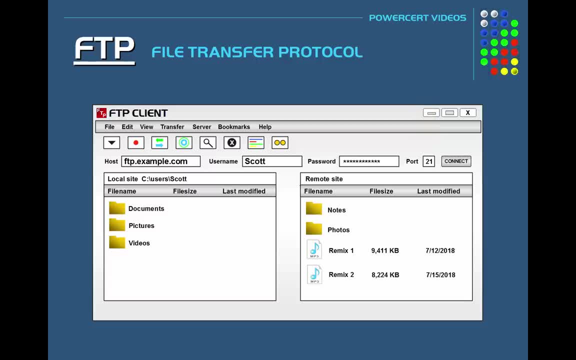 and now we're connected to the FTP server. So over here on the left pane you have the files and folders on your local computer, And then over here on the right pane you have a view of the files and folders. that's on the. 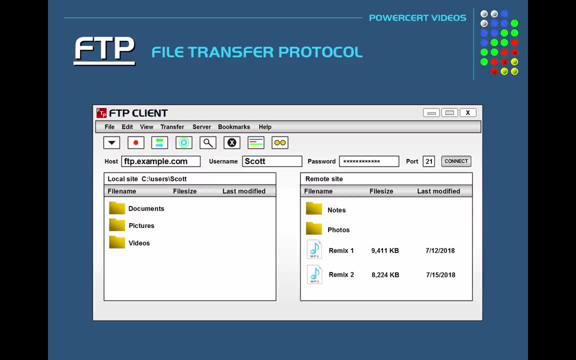 remote FTP server And then from here you can just click or drag and drop files from the FTP server, such as these mp3 files, and then download them to your computer just by clicking on them or dragging them over from the right pane to the left pane And if you have the proper permissions. 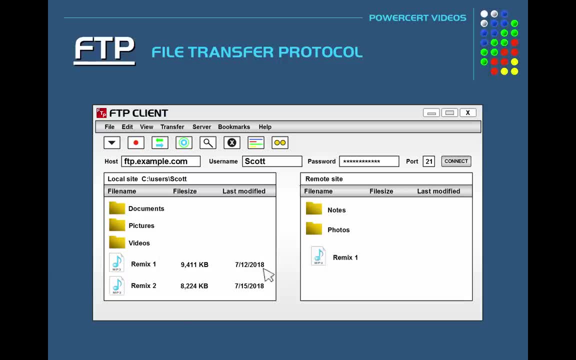 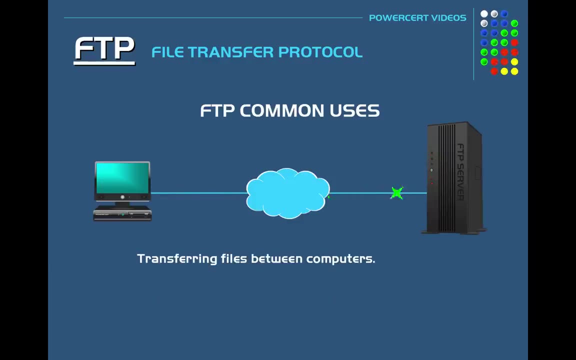 you can also upload files from your computer to the FTP server By dragging them from the left pane to the right pane, and then the files will be uploaded to the FTP server. So transferring files between computers is a common use of using FTP, especially when you're transferring files in bulk. And another common use of using FTP is to 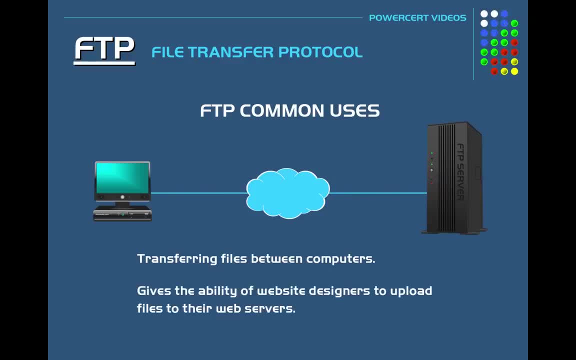 give the ability of website designers to upload files to their web servers. Now, the main drawback of using FTP is that it's not a secure protocol, So the data that's being transferred is not encrypted. All the data is sent in clear text, which can cause security concerns. So, really, 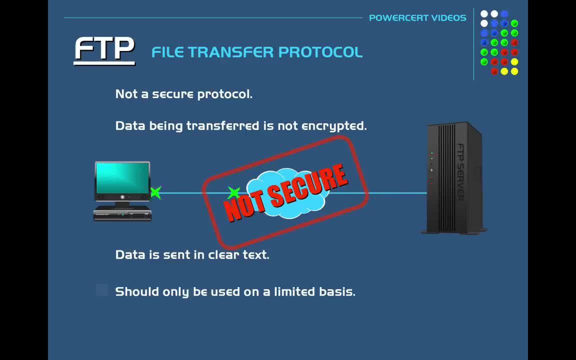 FTP should only be used on a limited basis or on only trustworthy networks, Or if the data that's being transferred is not sensitive. However, if you're going to transfer data that needs to be protected, a more secure transfer protocol should be used, And that's where SFTP comes in. 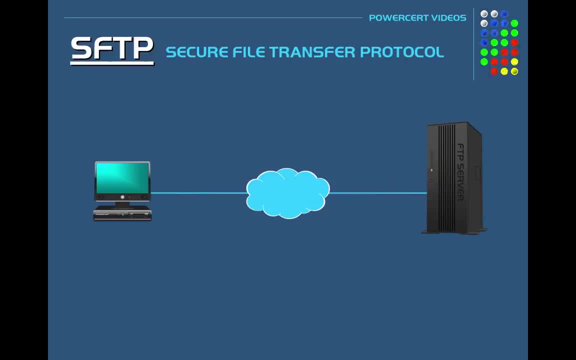 SFTP stands for secure file transfer protocol. Now, secure FTP is just like FTP, except that it adds a layer of security. The data using secure FTP is actually encrypted using secure shell during data transfer, So no data is sent in clear text, It's. 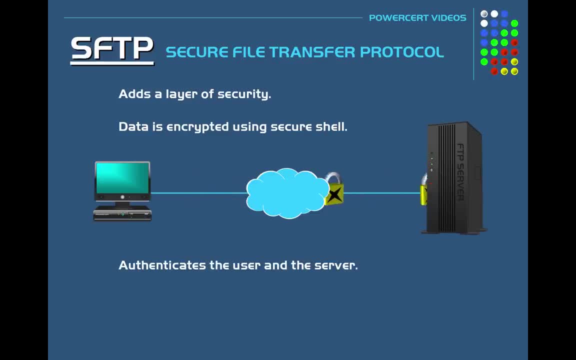 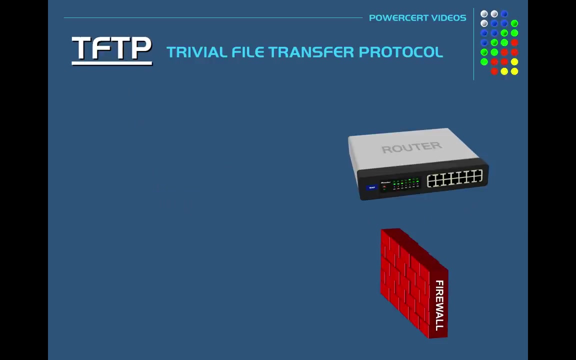 all encrypted, And secure FTP authenticates both the user and the server, and it uses port 22.. It's also important to note that both FTP and secure FTP are connection-oriented protocols that use TCP for file transfer, So they guarantee file delivery. And finally, there's TFTP: TFTP.